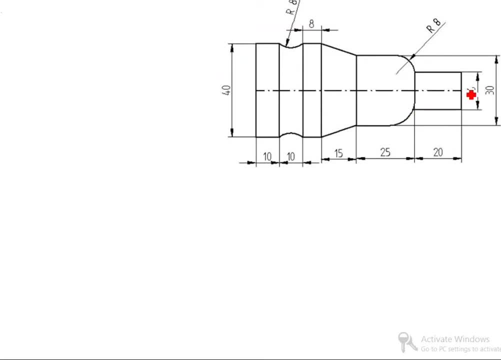 Today we will learn turning program. We will start from here. This is 0 comma 0.. This is plus z minus z. minus x plus x. So this is 0 comma 0.. So this is minus z. This is plus z. This is plus x. This is minus x. 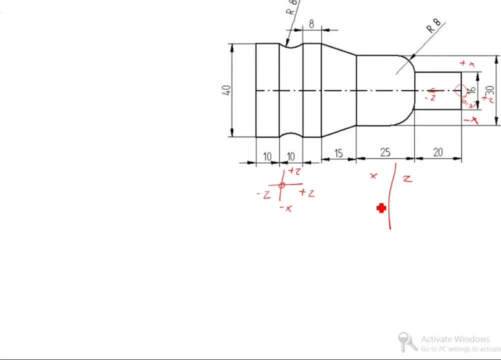 Next we will start x z values. x is 16. So you can write it 16.. z is 0.. So you can start 0.. Write it 0.. After that you see up to here is 16.. This value is 20.. So you can write 16 minus 20.. z is minus 20.. No minus, So minus 20.. 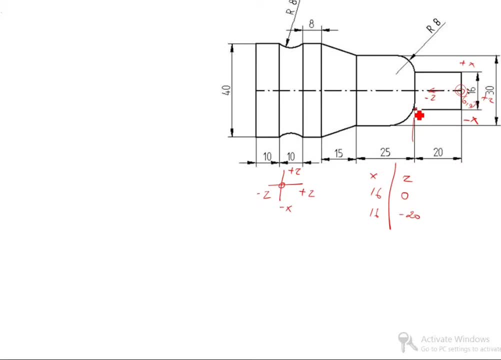 Up to here we finished. Here is r8.. r8 is radius 8.. So up to here this value is 8.. So this full value is 28.. z value is 28.. So x value is up to here. x is 16 only. 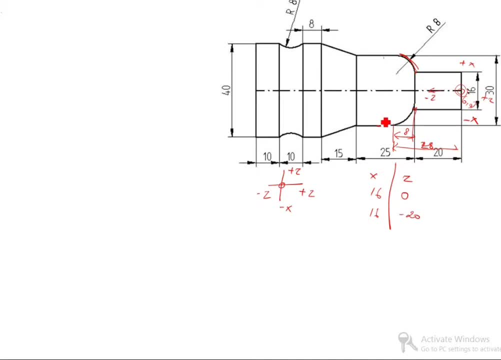 Up to here, the x value is 28.. 30.. Now up to here. we will see This is 16 minus 20. already wrote After that: this value is 30. This value is 28.. So you can write 30 minus 28 or 8.. 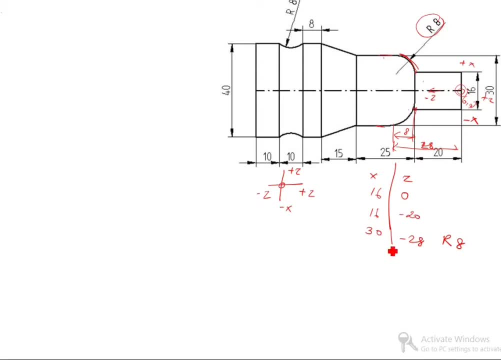 This one is given r8.. So r8.. After that, this full portion- up to here is 30. only This full is 20 plus 25, 45. So z value is minus 45.. x value is same, 30.. z value is minus 45.. Up to here, finished. 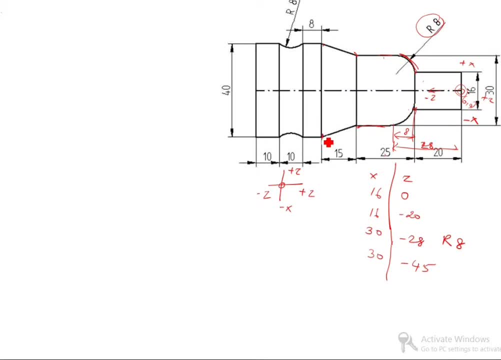 You go this side, What is this 40?? This is 40.. z is 45 plus 50, 60. So x is 40.. z is minus 60.. Up to here, finished, The whole thing is 40 only, So 40.. This is 8.. Up to here, So minus 60.. Up to here, minus 60 plus 8, minus 68.. 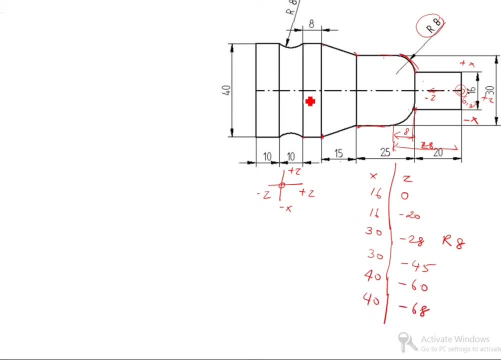 So 40 minus 68.. After that, you see, this value is r8.. But this value is 10.. x value is 40.. y value is not y value, z value. z value is minus 78.. Up to here, Minus 78 or 8.. 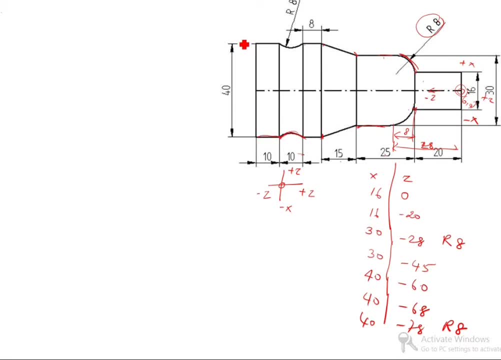 Up to here we finished. After that, the x value is 40. only Up to here. So x value is 40.. y value is minus 88.. Up to here is minus 88.. After final one, This is 40,. no, You can write it as 45 also. 45 means it comes this side. This way. This is the 45.. 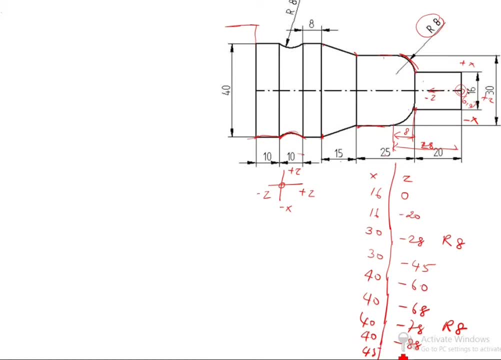 x value is 45.. z value is- I will write plus 3.. So this is 45 here. Plus 3 goes this side. So this way Plus 3.. So this is 45, comma 3, x value, x and z value. 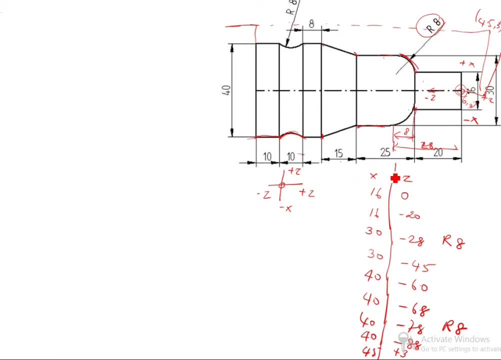 We have to remove the tool outside. That's why we have to write 45 plus 3.. We have to write 50 plus 5 also, No issue. Whatever number you have to write, you have to remove the tool outside. Okay, We have to write the program now. We will start from N11.. I will start N11.. Previous, we have to write it as N01. only Now we will start it as N11.. N21 also. you have to write 21,, 22,, 23.. We will start N11.. M012.. M012 is cramping the work piece. N12.. N12,, M06.. 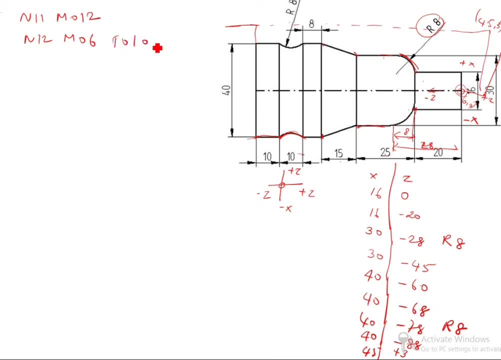 T0102. M06 is tool change. T0106 is tool number. We can write T0105 also T013. 03. also This is the tool number N13. M03.. This is spindle on, Spindle on Yes. 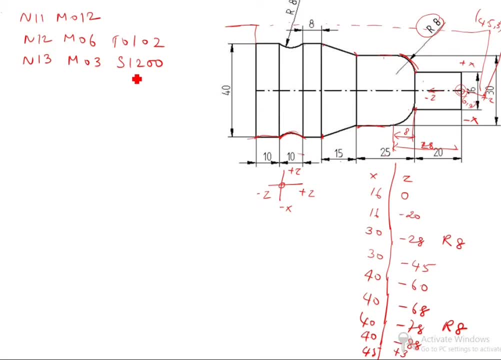 1200.. 1200, I will write, We will write. 1500, also 1000, also 600, also N14. M08.. This is coolant on N15. Z90. Z00. X0.. Is it 0?? 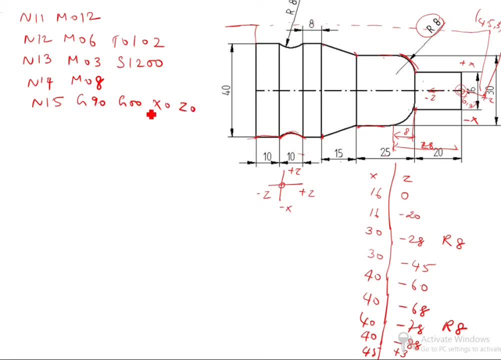 What is Z90?? Z90 is absolute program, Z00 is linear position. X0, Z0 is: we will start from 00.. Value is 00.. Start from 00, now 0, 0.. So that is why we wrote X0, Z0. 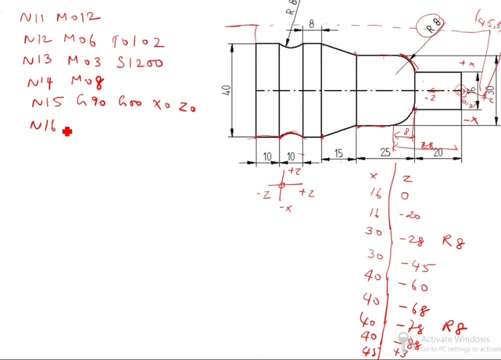 N16.. N16.. Z01.. X0, Z0. F5.. F5 is feed rate. Z01 is linear interpolation. The tool is in the linear motion only, So we will write Z01.. N17.. N17 is torque sub program. We will write Z01.. What is Z01?? X value is 16.. What 16? Plus 16.. So X16. 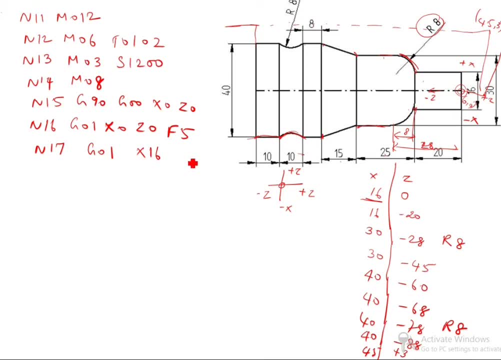 Z is 0.. You can write Z01.. also, it's not no value, no, so you have to remove that n 18. what is n 18? n 18 is z 0, 1 z minus 20. why is it minus 20? you see, 16 is there, this 16 is there, so don't write 16 again. 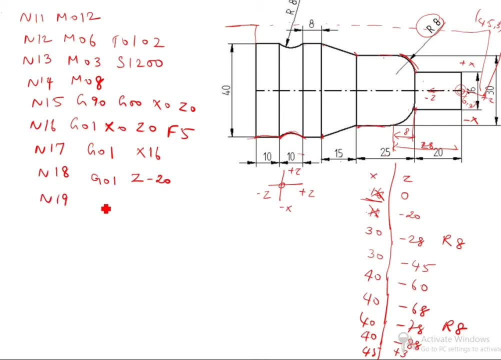 so minus 20, n 19, n 19 is. you see, this is portion, is upside, so upside is anti-clockwise. so anti-clockwise means z 0, 3. clockwise means z 0, 2, so anti-clockwise means z 0, 3. clockwise means z 0, 2, so anti-clockwise means z 0, 2. 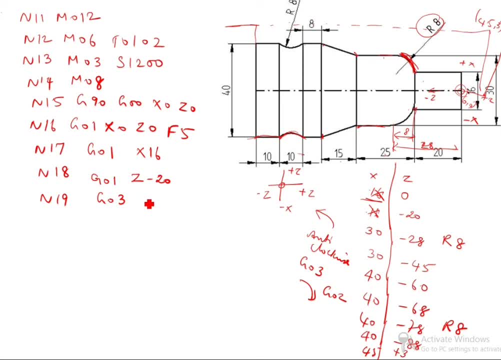 we can write g, 0, 3 X, 30, is it minus 28 or 8 up to here? is it after that n 20, z 0, 1, 30 already wrote, so don't take, don't try it again. so is it minus 45 after that n 21. 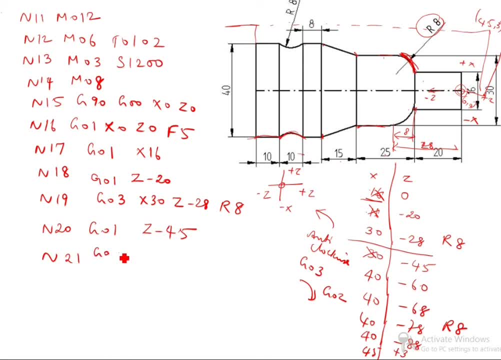 1, z 0, 1, x 40, z minus 16, n 22, z 0, 1,. all is x 40. now, If you write, also no issue, if do not write, also no issue, we have to write it here: x 40, z minus 68, n 23, z 0, 1, x 40,. 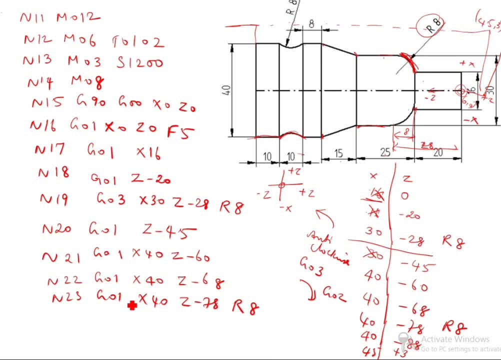 z minus 78 or 8.. You see, this is comes this way. no, this way. So this way means this one is goes here, this is clockwise. So this one you can write z 0, 2, n 24, z 0, 1,. 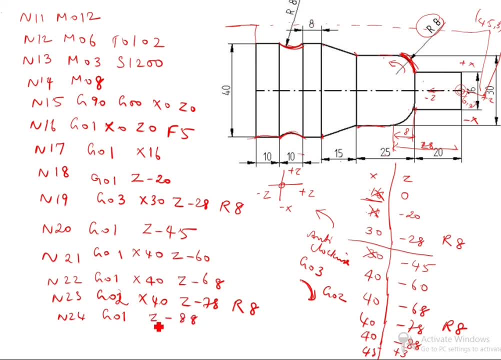 z minus 88.. Otherwise you can write x, 40, z minus 88.. Otherwise do not write x 40. also, you see, already is coming 40,, 40,, 40,. no, So do not write again n 25,, z 0,, 1.. 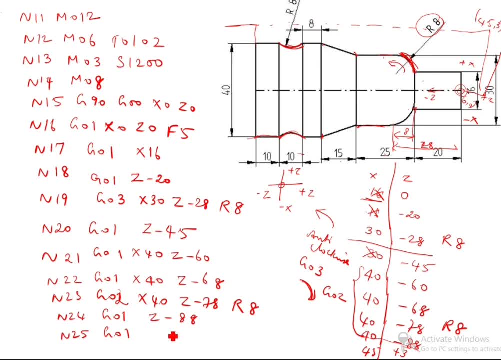 Now up to here, finished After that. final one is z 0, 0, x, 45, z plus 3.. N 26, m 0, 5.. What is m 0, 5?? M 0, 5 is spindle off After that n 27. M 0, 5.. n 0, 5, z 0, 1, n 2, 1, 1, 1 of those are send to off To make it perfect. we can write- speed is straight forward: 1, 1, z 0, 1, n 0, 1, z 0,. 2,, 1, x, 40, z l minus 8 or 9, z minus 8, z minus 8, z plus 3.. Now it is also general expression. You see, you have to do that only steady друзья. z 0, 1, z minus 8.. That always it is a should be+, and if you say it is, then it is skip that you have to read these: R z z minus 8.Now let us do another step.